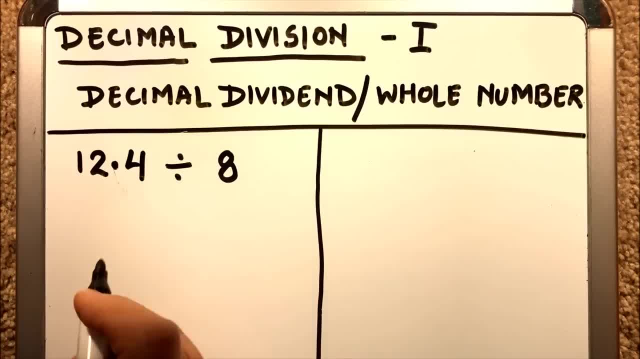 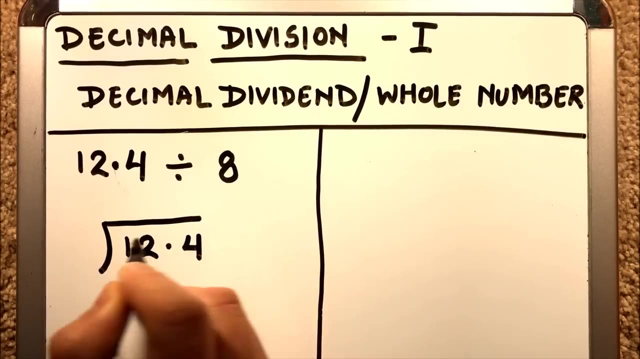 So decimal division: we'll start it as a normal division, but we need to take care of the decimal point here. So what we'll do? we'll put the decimal in the quotient just above the decimal point in the dividend. So I'll show you how we do this. So we'll write it as is and then we'll divide it by 8.. 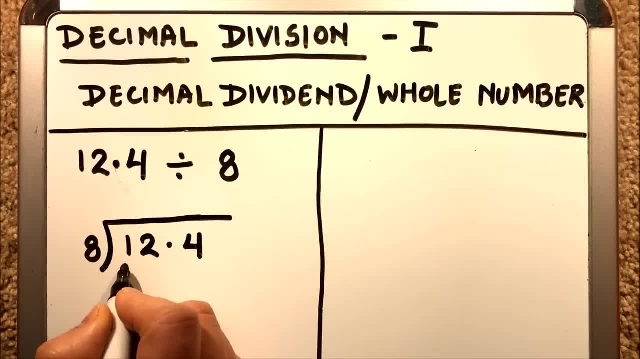 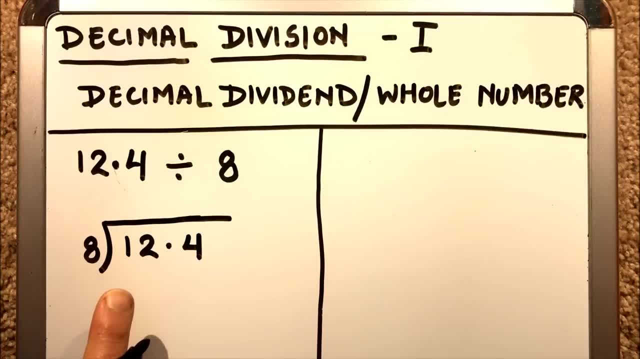 So first we'll check the height. Highest decimal place Here: 1 is the highest decimal place Here. we see that 1 is not divisible by 8 because it is very less. So we'll take two numbers together, So 12, we'll divide 12 by 8.. 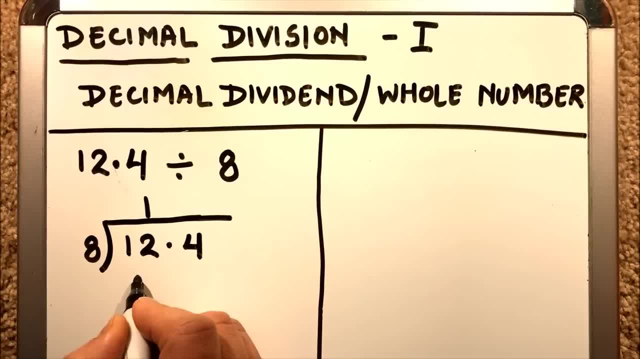 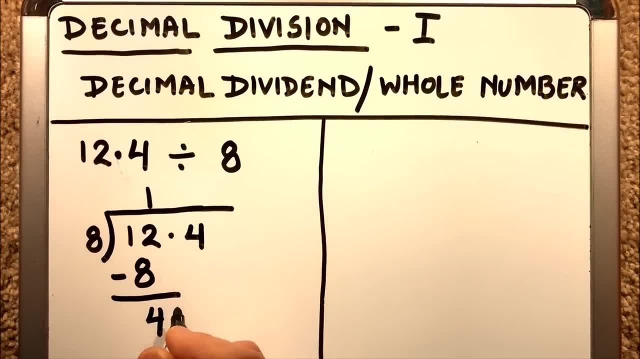 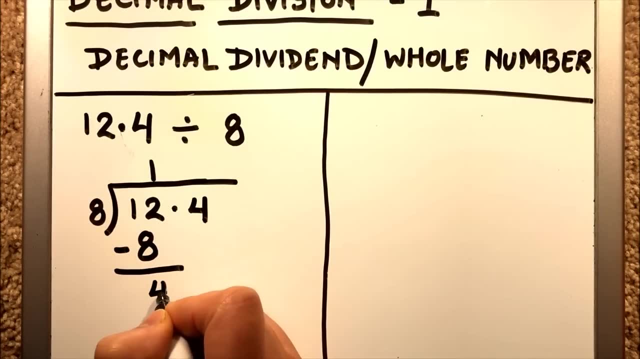 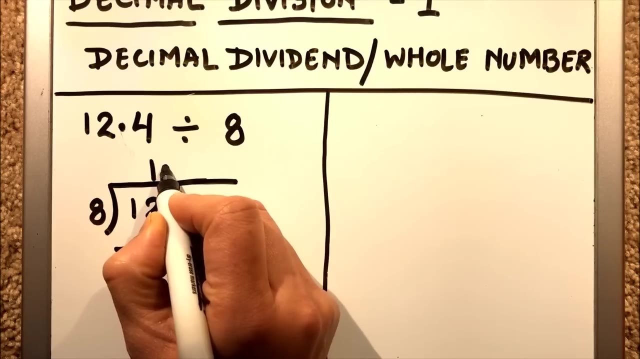 So we'll count the tables of 8.. So 8 times 1 is 8.. So we'll get the remainder 4, and then just above this decimal point in the dividend. Now We'll get 4 and in the remainder and we need to drop the next number. But in between there is a decimal point. So we'll put the decimal point in the quotient as just above the decimal point in the dividend. 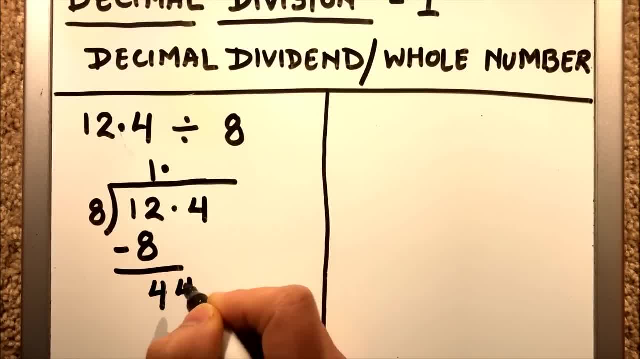 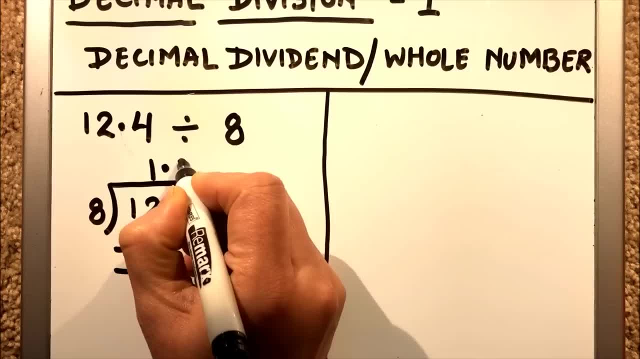 And then we'll drop down the next number, which is 4, here, And then we'll count the decimal, We'll count the tables of 8.. So tables 8 times 5 is 40.. So this is 4, 0.. 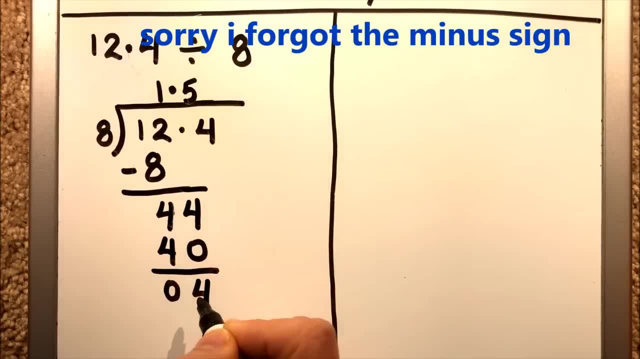 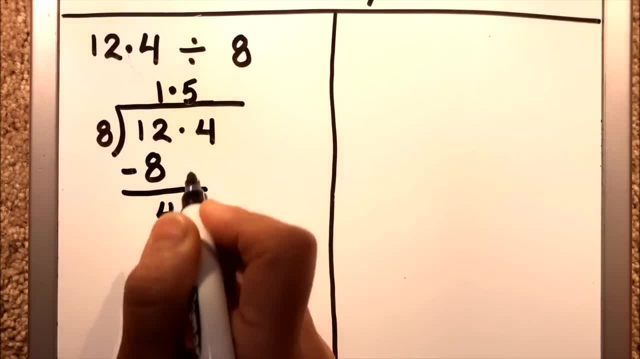 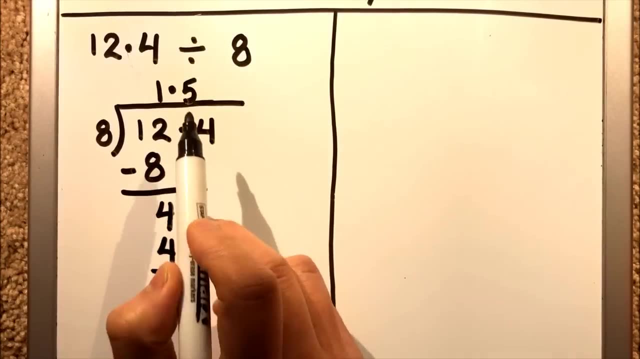 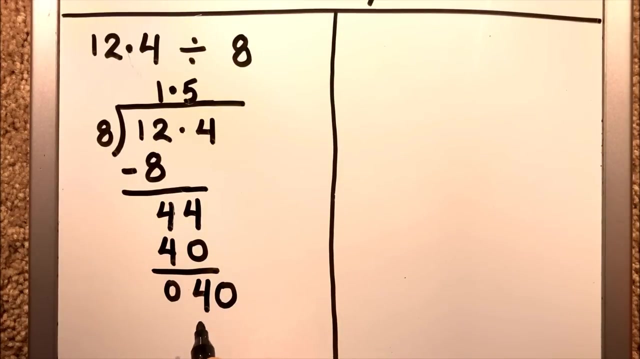 And then this is 0. This is 4.. Now this 4 is the remainder. If there is a remainder, what we'll do is we'll write a 0 to continue the division. So because we have already put the decimal point, so we can write the 0 in decimal division, not in normal division. In normal division we can't put the 0. We need to put a decimal point for that. 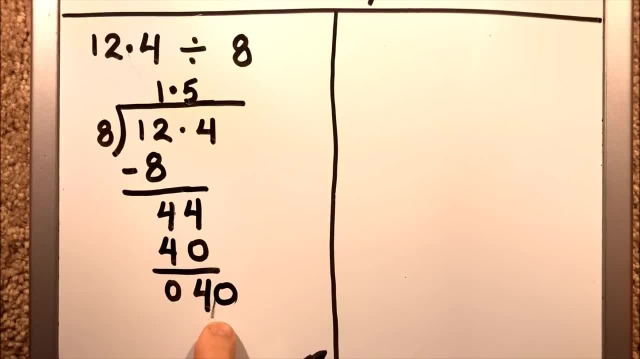 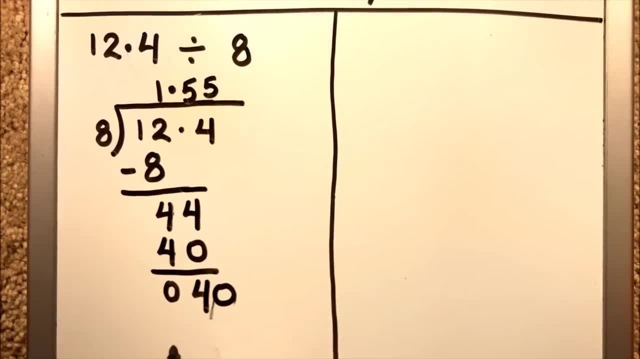 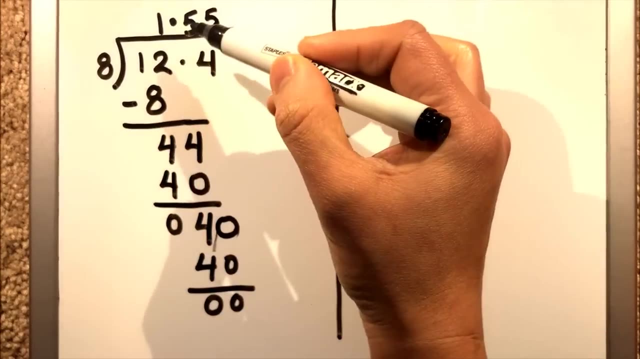 So here we are doing decimal division, So we'll put the 0 here And then we'll count the decimal. We'll count the tables of 8, which is 8 times 5 is 40. So this will be 4, 0,, 40.. And the remainder is 0.. So our quotient is 1.55..